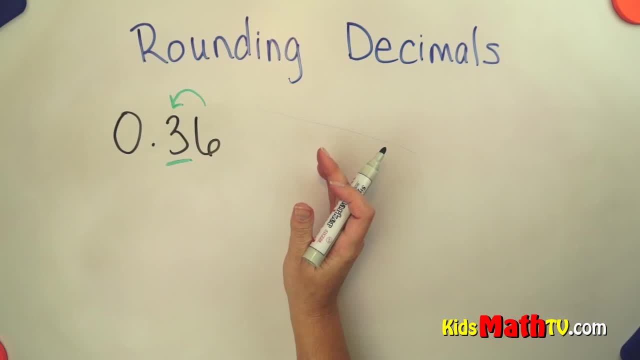 to do whether it's going to stay a 3 or move up to a 4 tenths. So it's either 0 and 3 tenths or 0 and 4 tenths. The rule is, if this number is 5 or greater, it makes this number move. 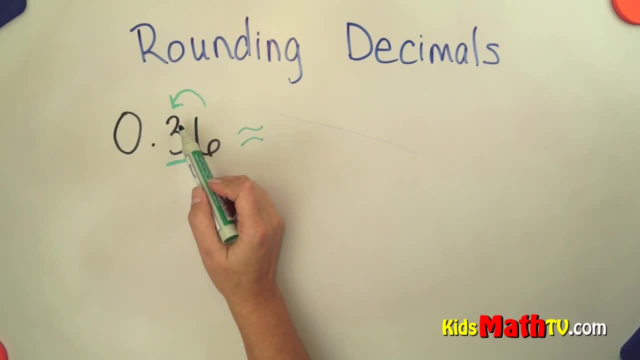 up one. If it is 0 to 4, this number stays the same. So since this 6 is 5 or greater, it's telling this number to move up one tenth, Because this is actually closer to 4 tenths than it is to 3 tenths. So our answer is 0 and 4 tenths. 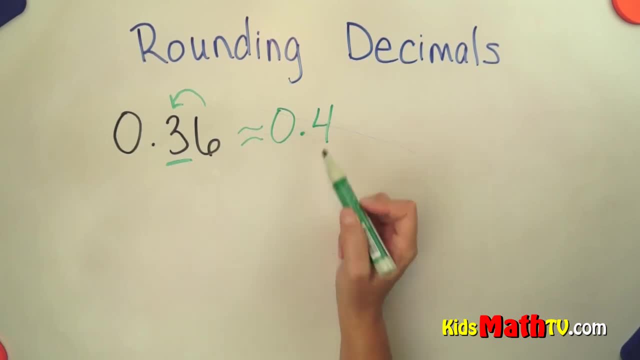 So 36 hundredths rounds to 4 tenths. Let's try another one. So how about 4 and 521 hundredths? Sorry, 521 thousandths, but we are going to round to the hundredths place. So the 2 is: 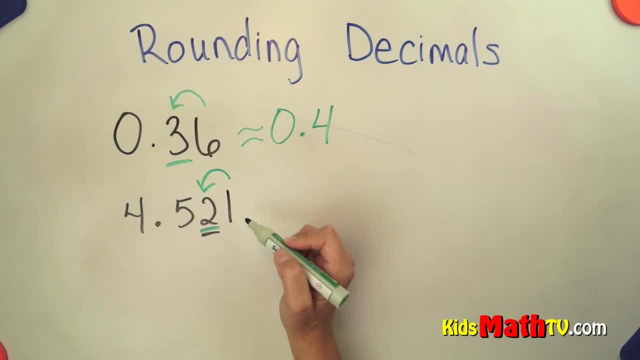 in the hundredths place. This 1 tells this 2 what to do. Is it going to stay the same or go up to 3 hundredths Between 0 and 4.. So this number is actually going to stay the same, So this will be 4. 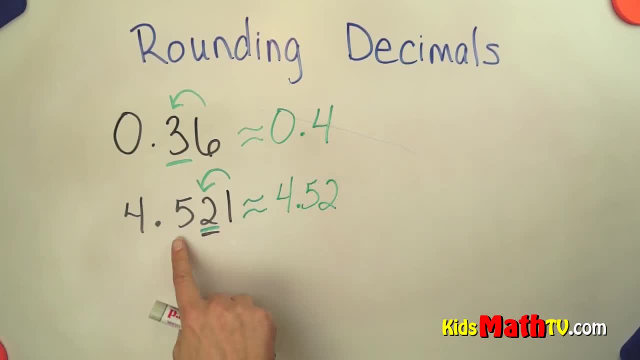 and 52 hundredths. This is closer to 52 hundredths than it is 53 hundredths. How about one more About 36 and 9 hundredths? no, 9 thousand, 9 hundredth, 95,, 10 thousandths. 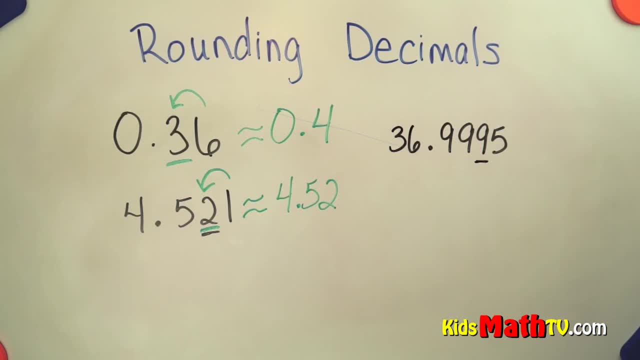 And then we are going to round to the thousandths place. So this 9 is in the thousandths place. This 5 is going to tell that 9 what to do. This is a tricky one. So this is either closer to 36 and 9 hundred and 99 thousandths, or 37 whole. 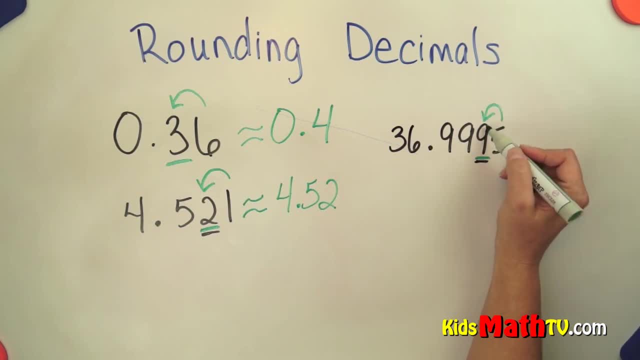 So, in this case, this tells this up to this. 5 tells this 9 to go up 1 to 10, which makes this go up to a 10.. makes this go up to a 10,, which makes that go up to a 7.. So this actually, 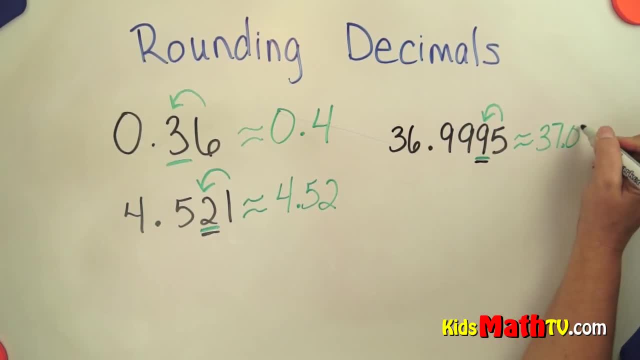 rounds to 37 and 0 thousandths. Those are tricky with the nines, And that's the end of our lesson on rounding decimals. 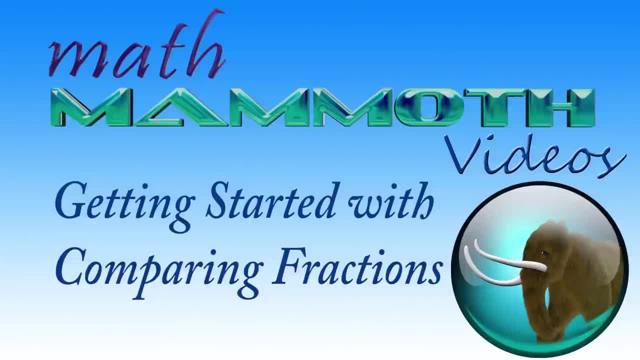 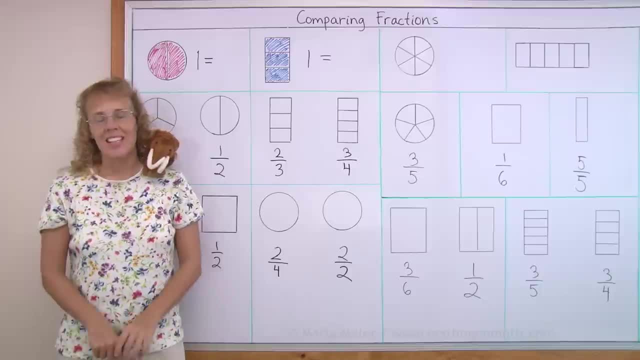 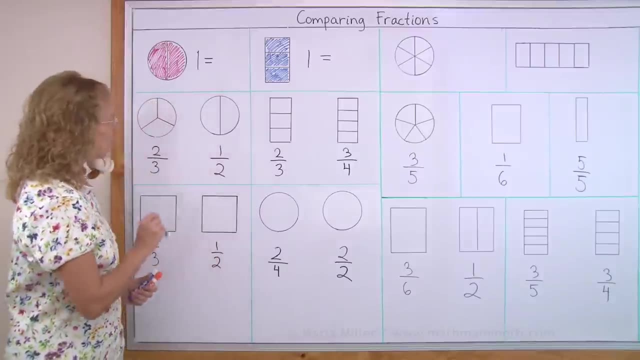 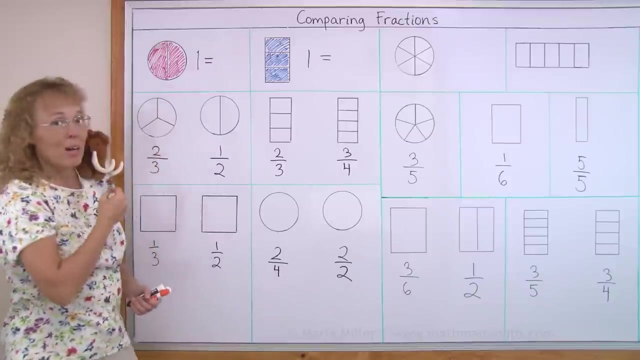 Hello, my name is Maria and this is Matthew, my mascot. In this lesson we are going to compare fractions, Try to find out which fraction is greater. But first, before we get into comparing, we are going to just review something important, which is here. I have one whole 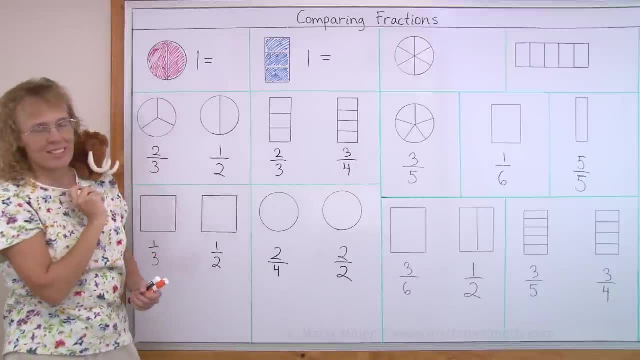 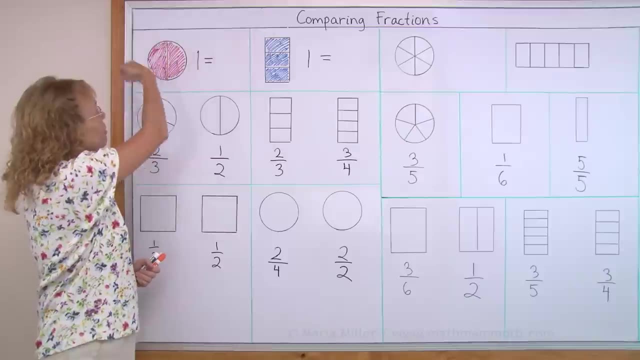 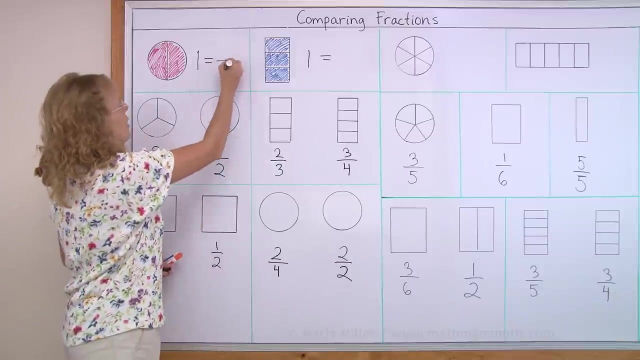 circle, but I divide it into two parts, and both parts are colored. What fraction is it there for? I wrote here one, because it's one whole, but we can also write it as a fraction, And since there are two parts, then it is two there, and since two are colored, two. 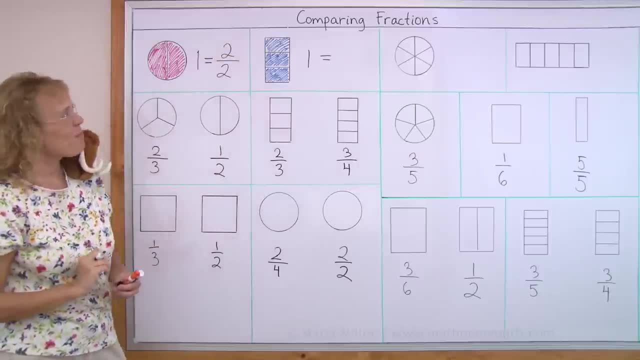 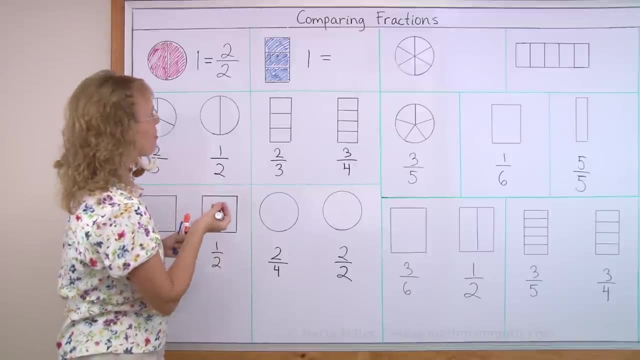 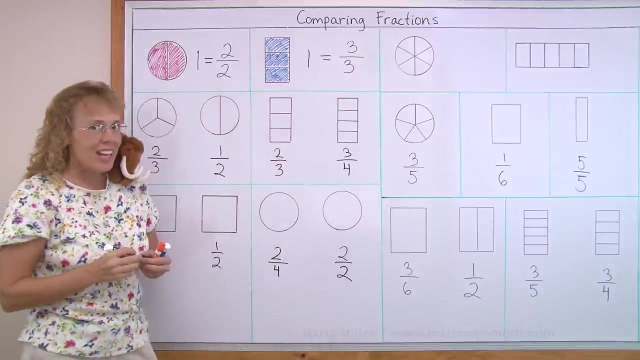 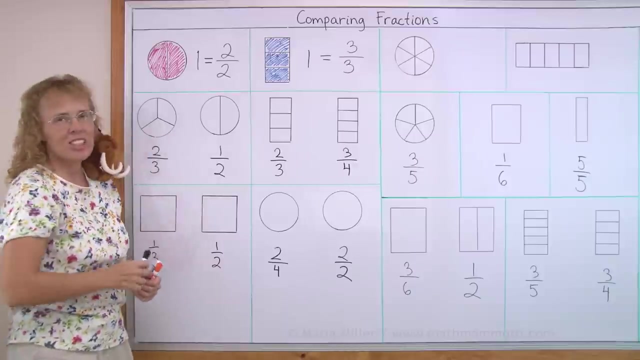 here too, And we read it as two halves. How about here? There's one whole rectangle, and how do we write it? We write it as a fraction, As you can see, three parts in total, three are colored, and we read it as three thirds. And over here we get to comparing fractions, which is kind. 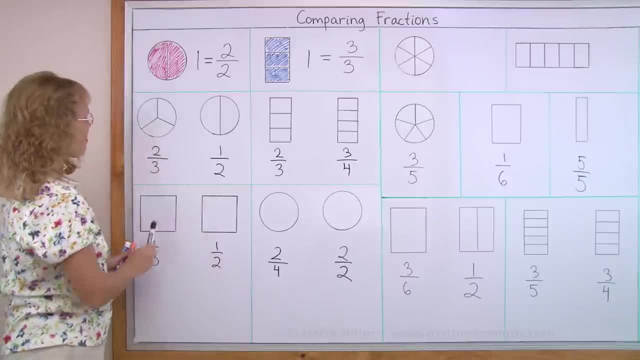 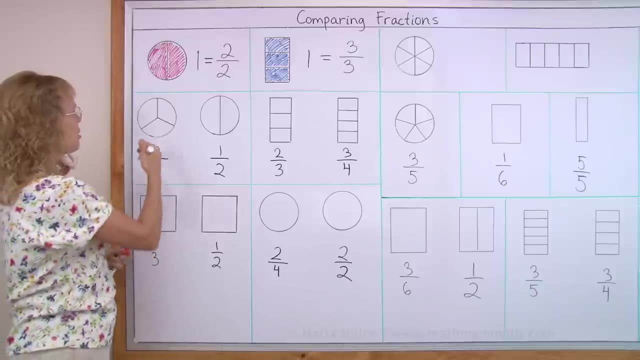 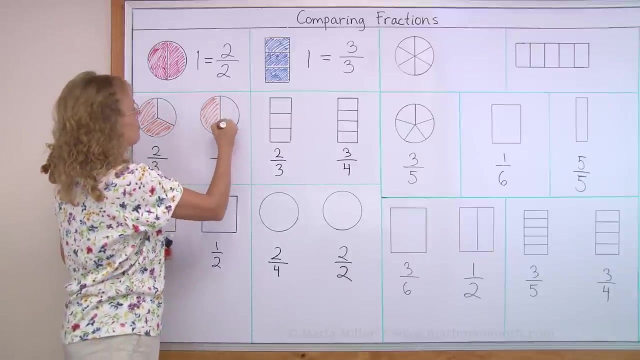 of fun because you get to color. Okay, what fraction is this? Two thirds, And that means I would color two of these parts here And over. here we have one half, so I color one part And now we compare which is greater. 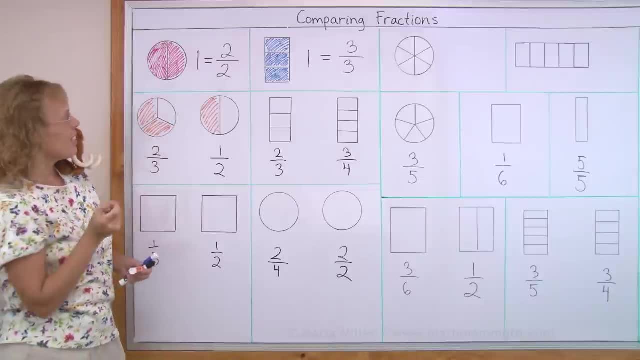 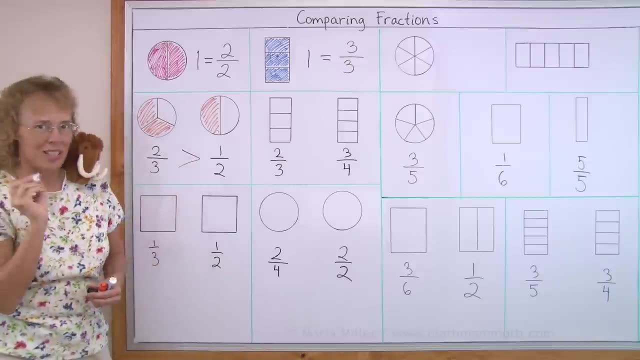 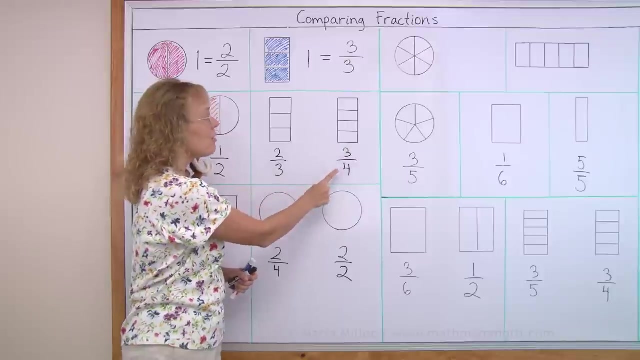 Which is more pie to eat, so to speak. You can think of it as a pie, you know, And so you see. oh, this is more right. So the alligator mouth goes that way Over here. two thirds, and what fraction is this? Three, fourths. So I need to color again.